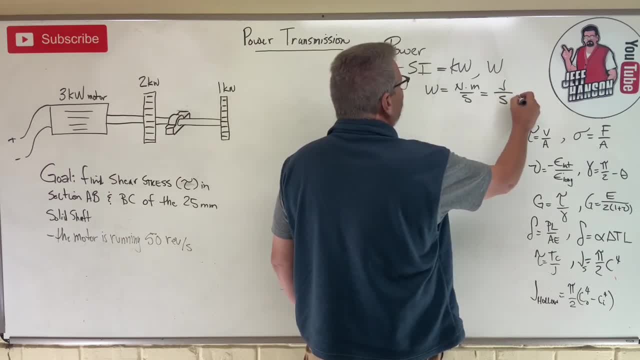 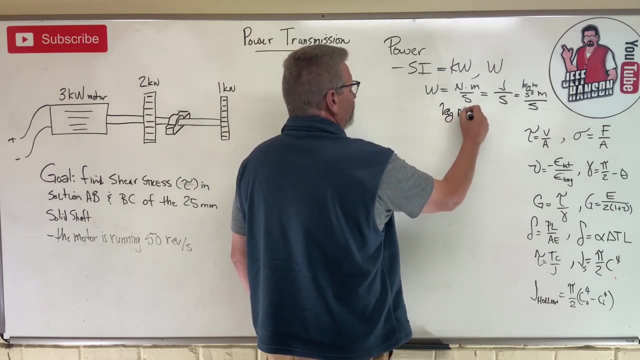 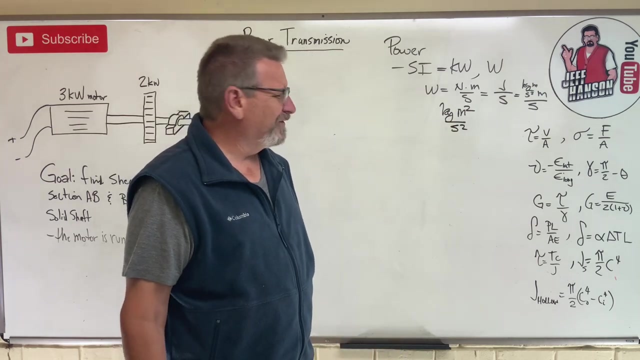 well, you could really get on down with your units and say, okay, a newton is a kilogram meter per second squared, Times meters, times seconds, which would give you what is that? A kilogram meter squared per second squared. When would you ever use those units? Well, I don't know, Maybe you're given. 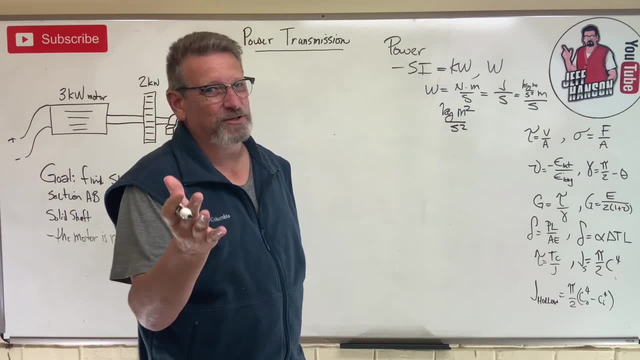 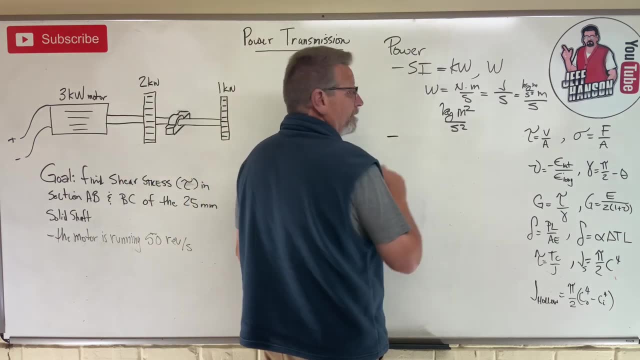 something and you need to make sure your units cancel out. You know I've been preaching to you about canceling your units out, So important, right? So there you go for SI And then, of course, for freedom units. Okay, 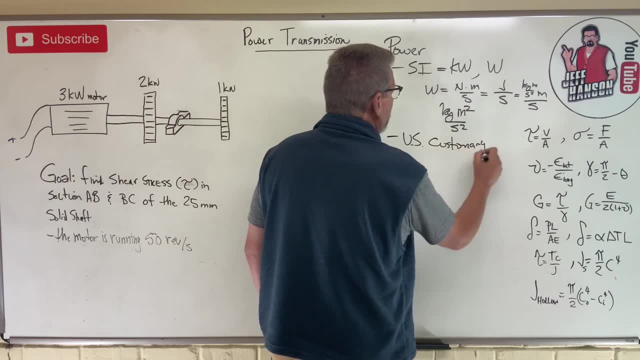 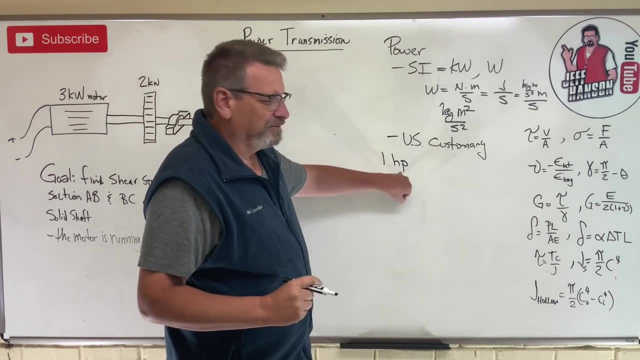 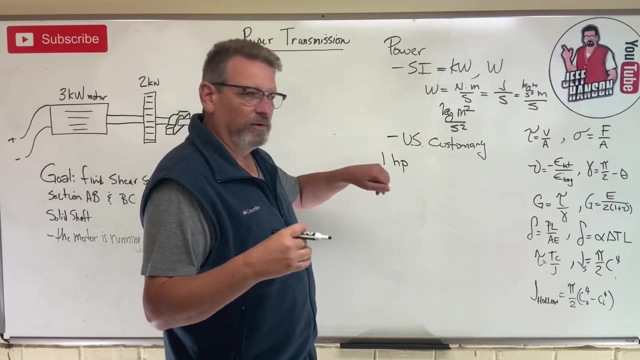 This is customary. Okay, We have one horsepower right Which was invented by a guy that came up with an engine for a car and he needed a unit to say: how good is my car? It will, you know, outperform. So then, once he came up with the horsepower as a unit, he had to go find some. 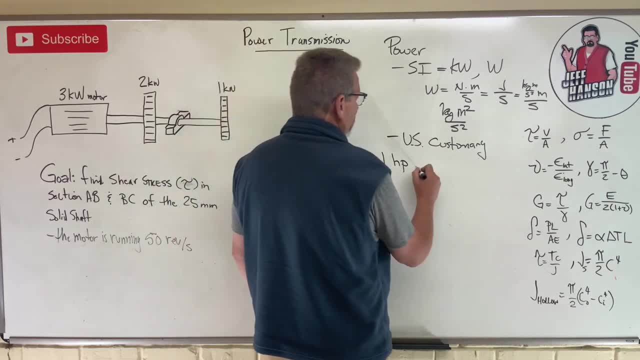 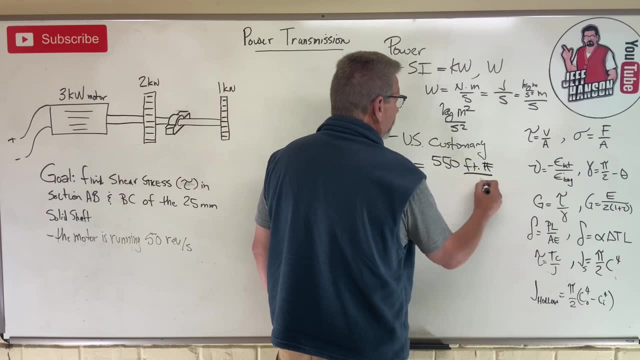 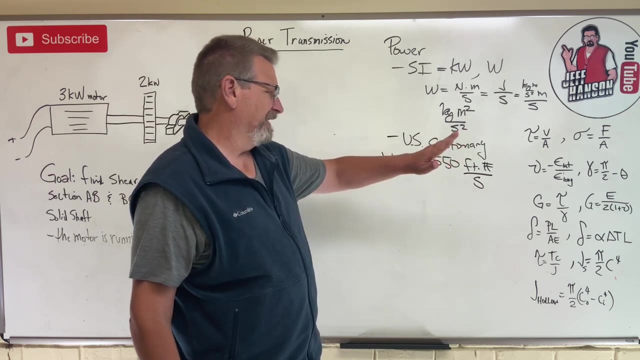 way to quantify what was a horsepower. But over the years a horsepower has become, I don't know, a very common thing. But anyway, we're going to divide this by 50. So we're going to divide this by 550 foot pounds per second right. Forget about dividing stuff by 10, Mr 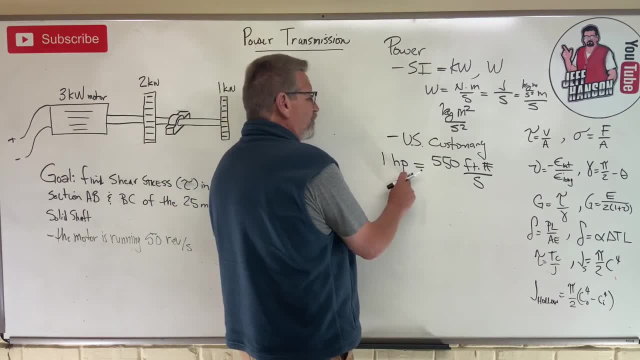 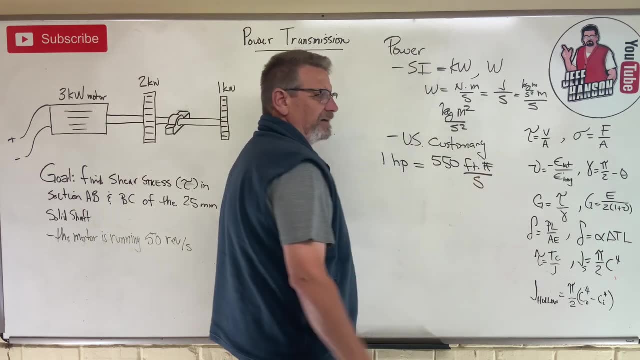 Metric Unit. We're going to divide by 550.. How about that? So, anyway, you're going to see horsepower given and know that it's foot pounds per second. Again, foot pounds work divided by seconds for time. Okay, What would take the horsepower to do that? Well, you know, we're going to divide this by 550 foot. 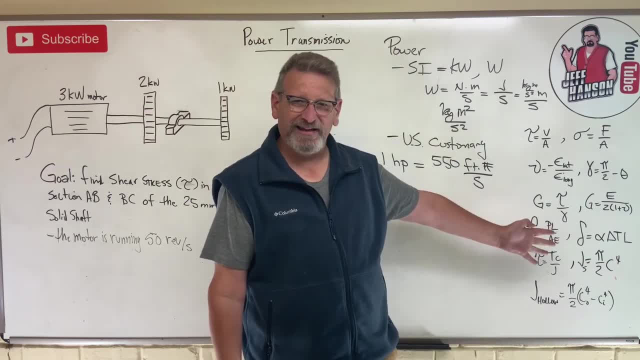 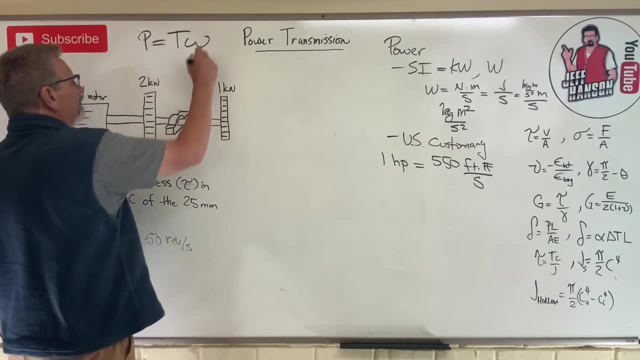 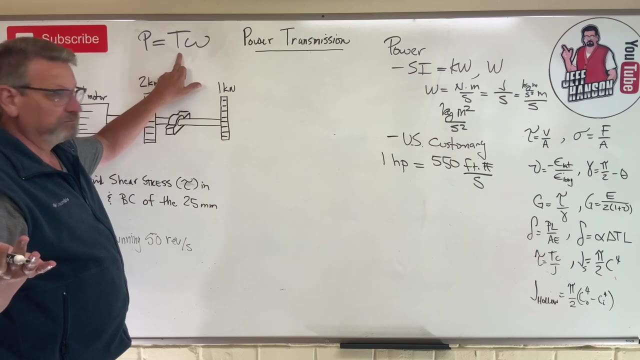 pounds per second. So what we're going to do is we're going to divide this by 550 foot pounds per second. Today's lesson B, without a brand new equation. Here we go. Okay, So power is equal to T times omega. Okay, P is for power. That's what power is T? torque, Torque, What is that? That's foot. 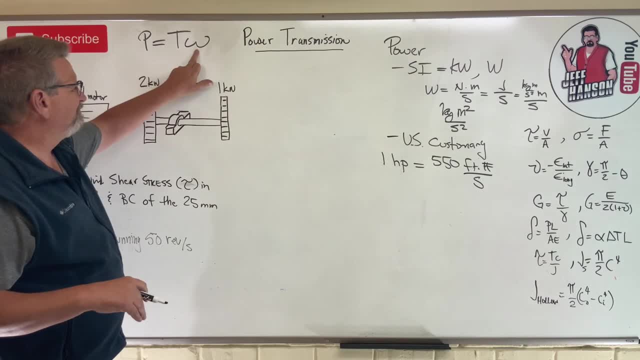 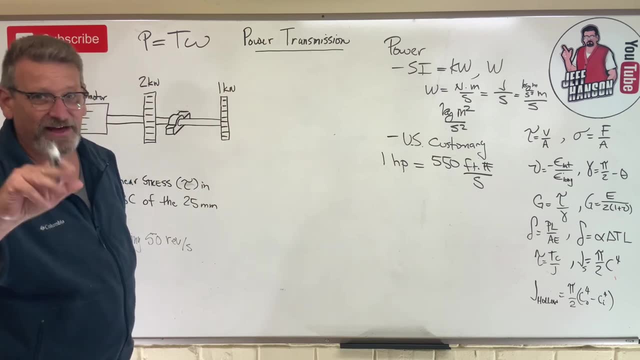 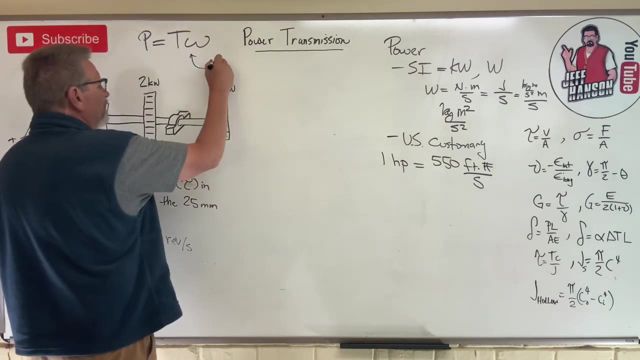 pounds or newton meters. And then you got this guy: new variable of the day. My students call this T booty. Okay, Now you get that out of your head. You get that out of your head. You get that out of your head. I dare you. Okay, You got this guy right here. omega- What is omega? Omega stands: 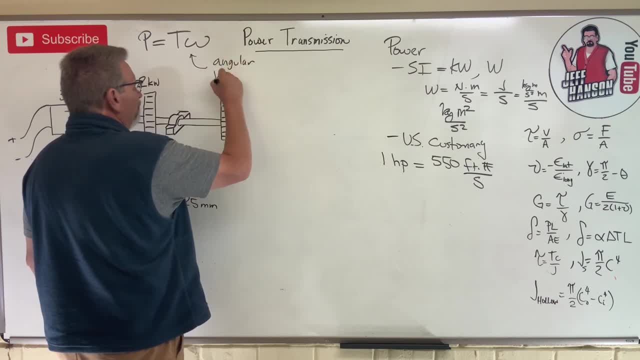 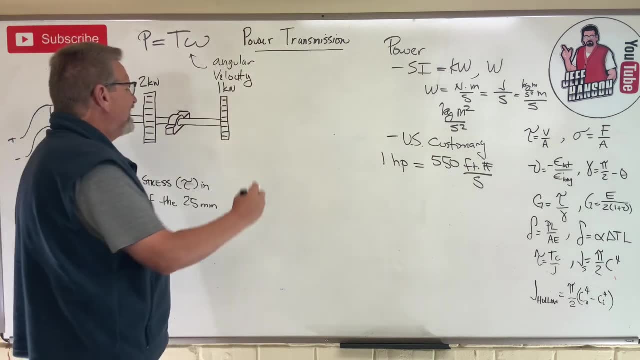 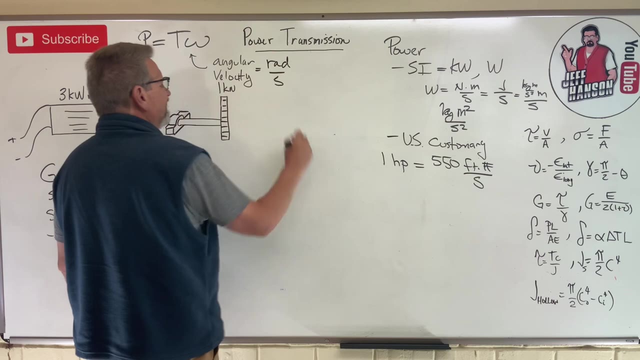 for angular velocity. Okay, And how does angular velocity need to come? It needs to be in these units. It needs to be in radians per second. Okay, That's what your goal is. If I give you an equation, I'm going to change it, I'm going to change it, I'm going to change it, I'm going to. 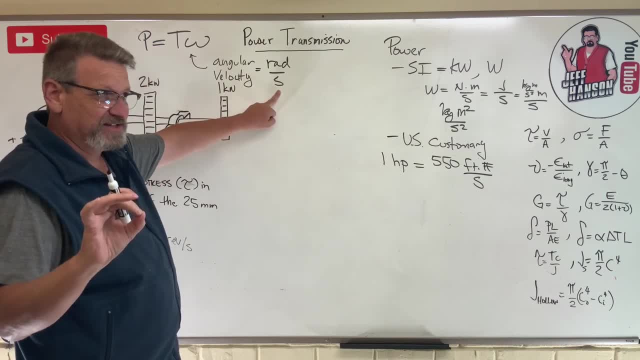 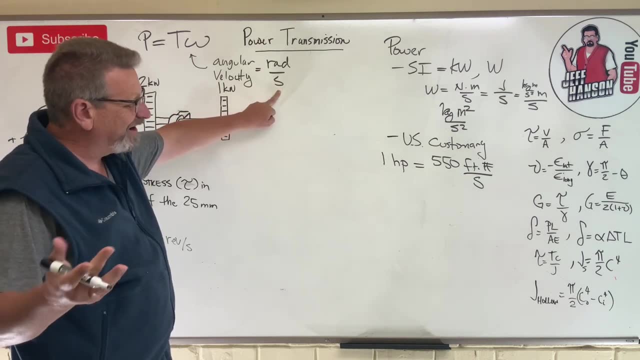 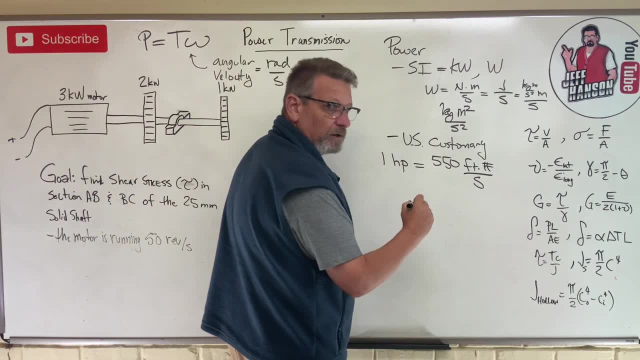 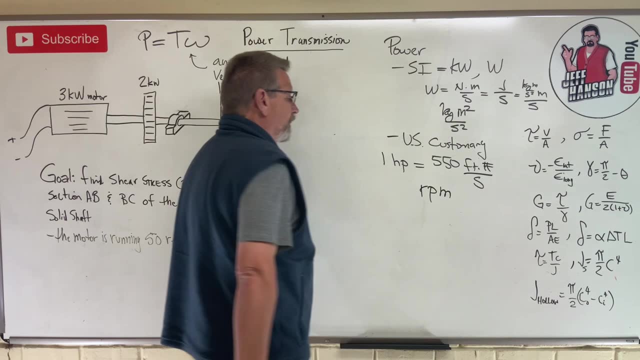 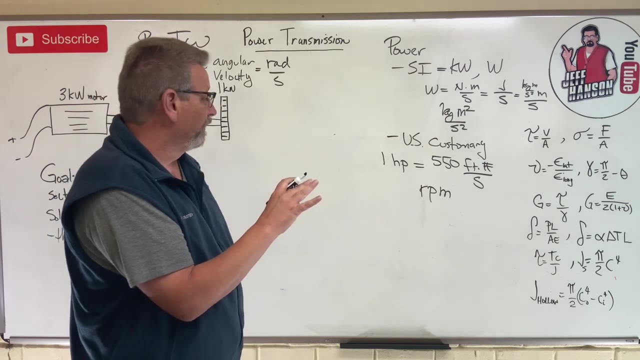 well, I could give it to you. oh sorry, what is wrong with you today? I could give it to you in ribbons. RPMs, right? how do you get that? how would you get RPMs, which is a very common way to express angular velocity? is this a revolution? 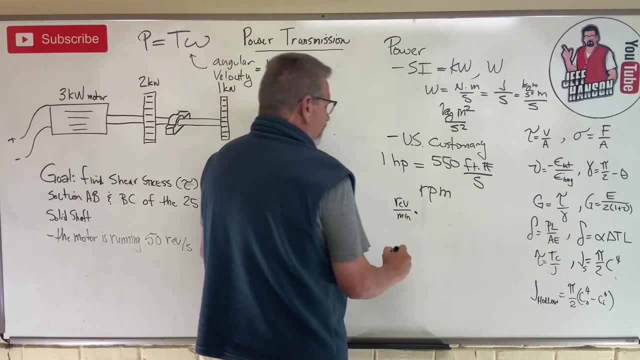 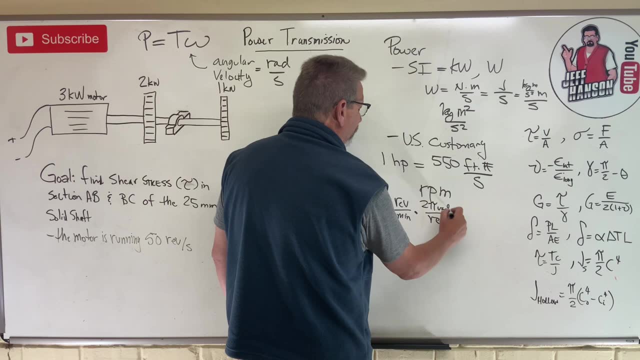 per minute. okay, let's see, I gotta get rid of that revolution. so I'm gonna put a revolution on the bottom and there's two pi radians in a revolution and then I need to get- remember, I need to get radians per second. so I get it rid of. 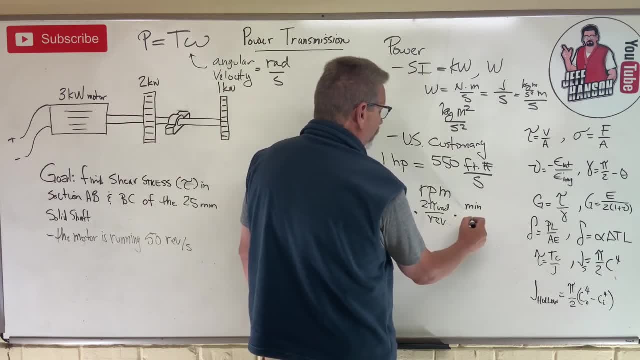 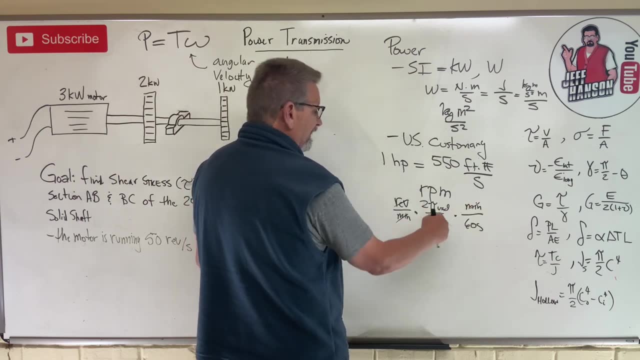 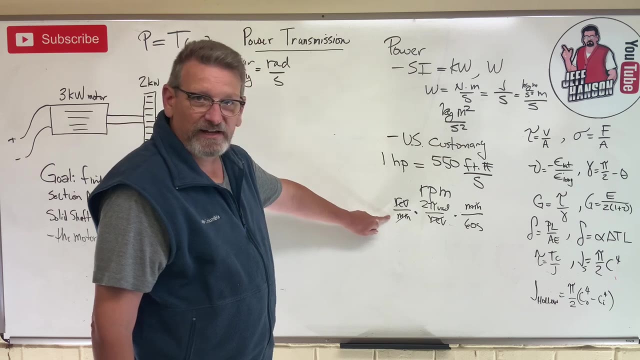 minutes. so I'm gonna put a minute on the top. and what do I have? 60 seconds in a minute. and so guess what revs cancel you, the men's cancel, and it leaves me with radians per second. so 2 pi divided by 60 will convert RPMs into radians per second, which is what I need, right, okay? 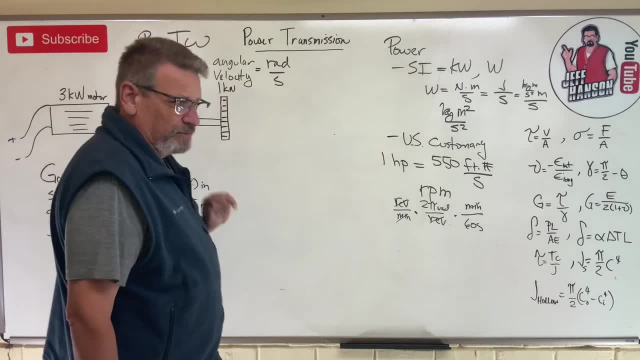 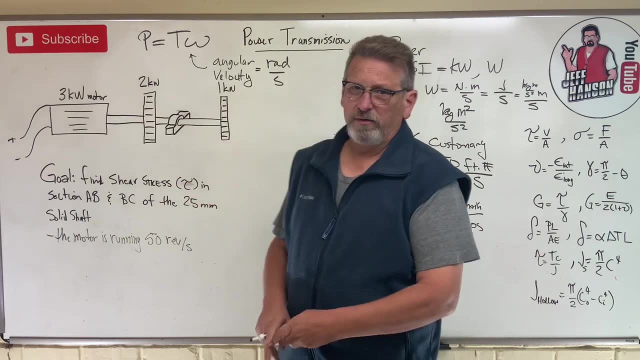 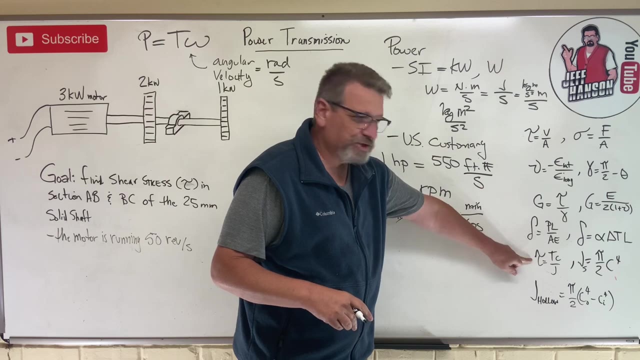 so there's our new equation and there's all of the terms in the equation. so what do we got here this time? we want to find shear stress, how that's for torsion. that's a twisting chef. it's rotating right. that sounds like sheer stress. sounds like that guy, doesn't it? 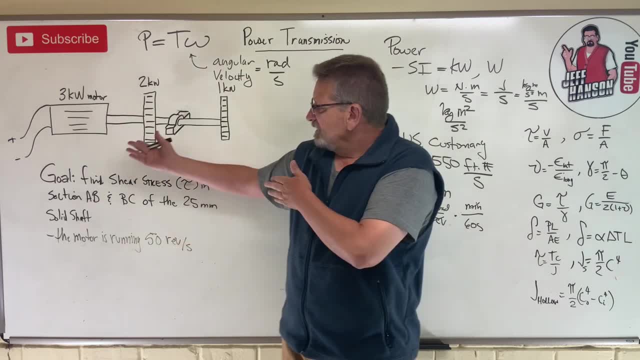 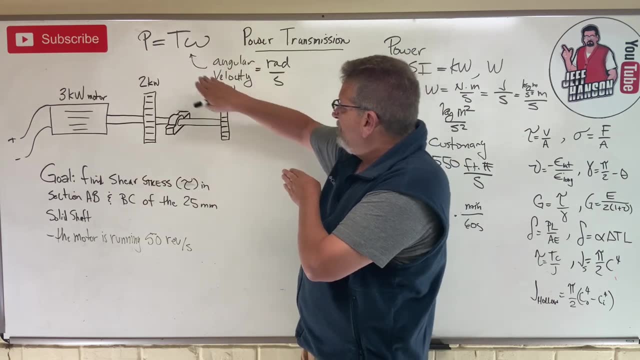 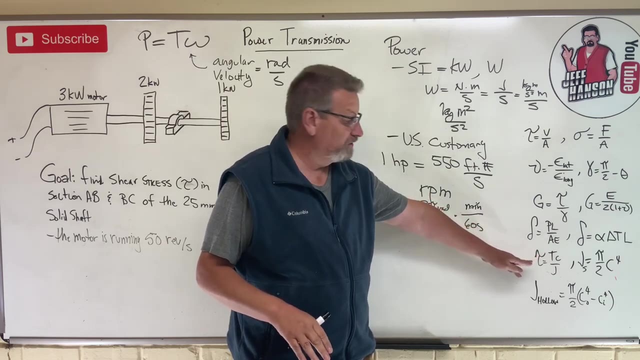 TC over J, but notice, in this problem they don't give me torque anywhere, right? so what we're going to do is we're going to use our new equation to back that guy out, to then go and substitute ba-BAM over there into that equation, right so? 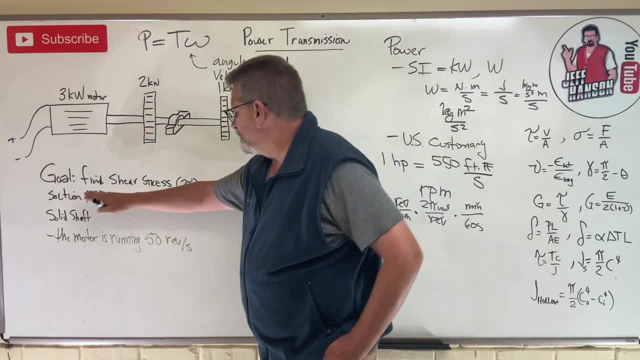 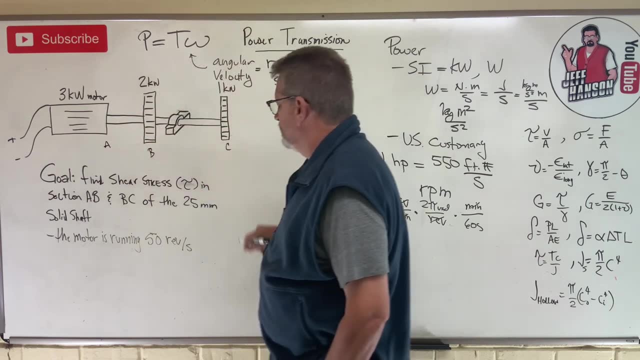 then we can get T zelf, which is what we need. so the goal: fine, shear stress, how in section AB? well, here's a, here's B here on the защ photography table. section AB will help me tighten 3 points tonight: Z, right over here, okay. and section BC. So what's going on here? What's going on there? 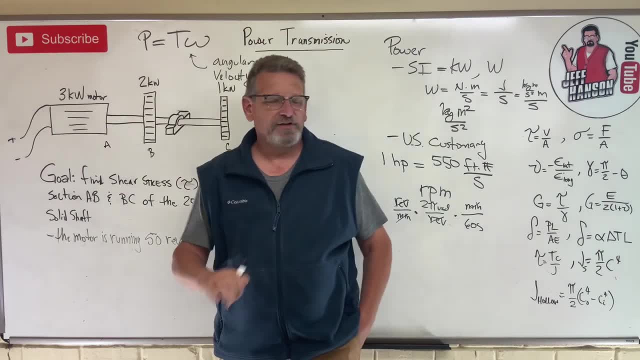 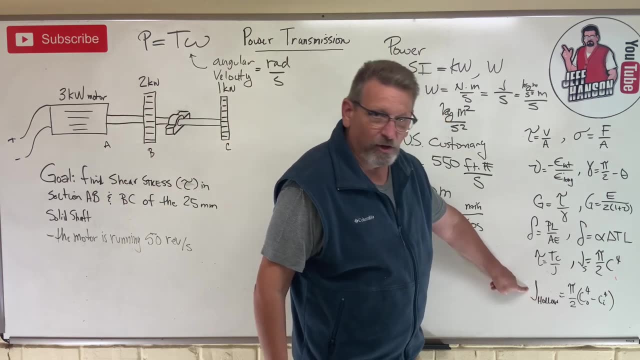 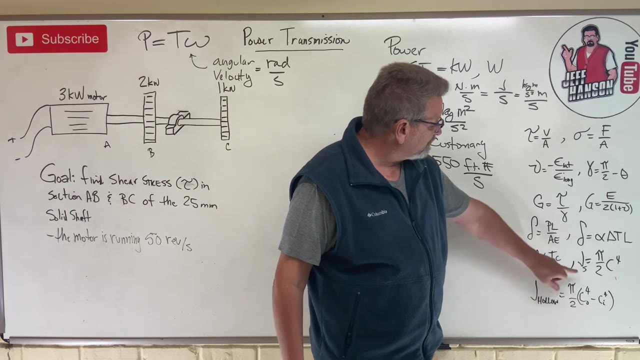 Of the 25 millimeter solid shaft. So remember, we got to find J and I have two equations. I wrote them both for us over here. Here's J for hollow, which is the outer radius minus the inner radius to the fourth. But that's for hollow. For solid, we don't have an inner radius, We just 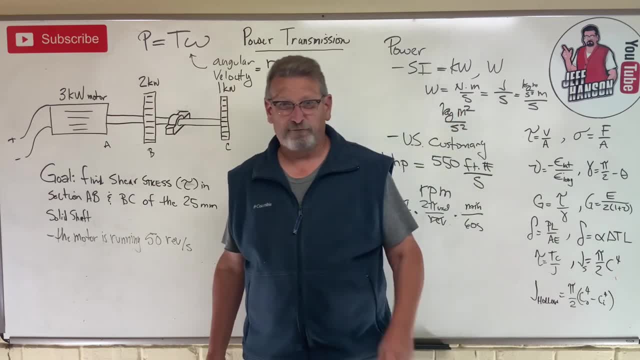 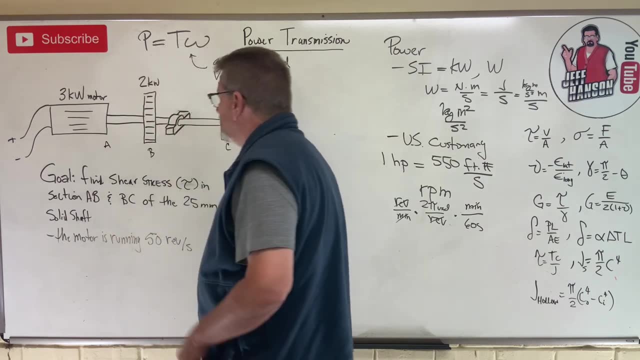 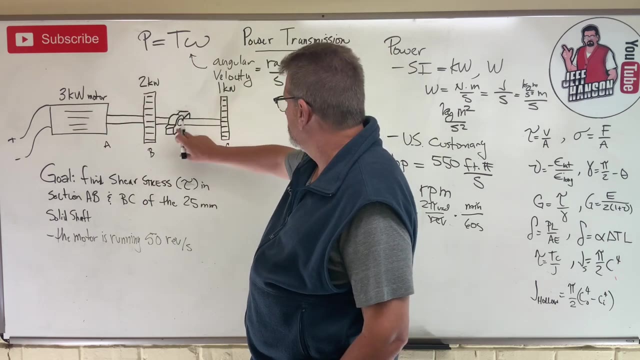 have an outer only. So it's just pi over two times C to the fourth. Remember that guy. Don't get J confused with I, right, Okay, so the motor is putting out three kilowatts. right, I've got a bearing over here, a pillow block, And what about this? Maybe this is like 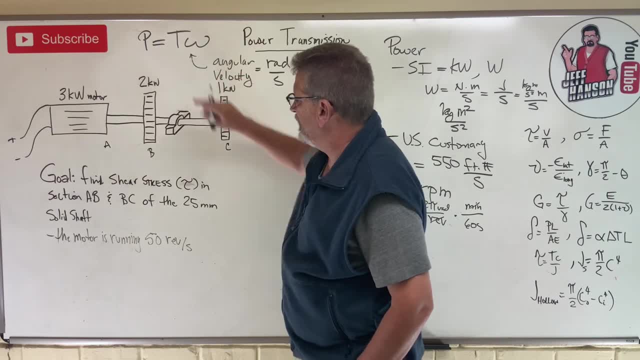 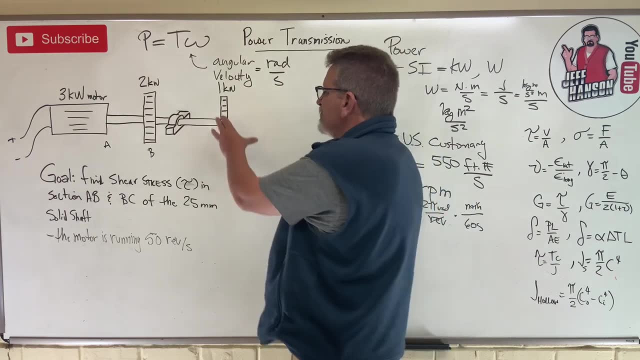 a big factory and there's a belt on this right, A belt on that, and it's taking off and this belt's driving one machine and that belt over there is driving another machine right, So this one is taking that's a W, for what one kilowatt of power That one over there is taking? 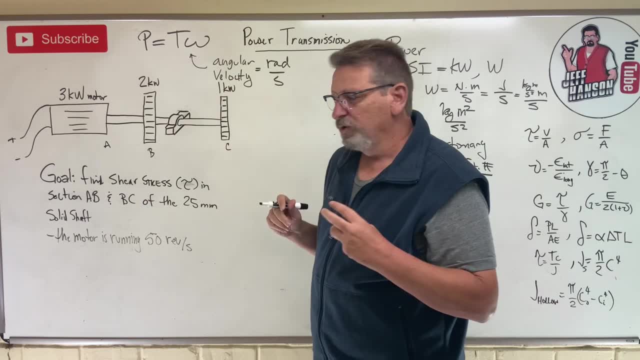 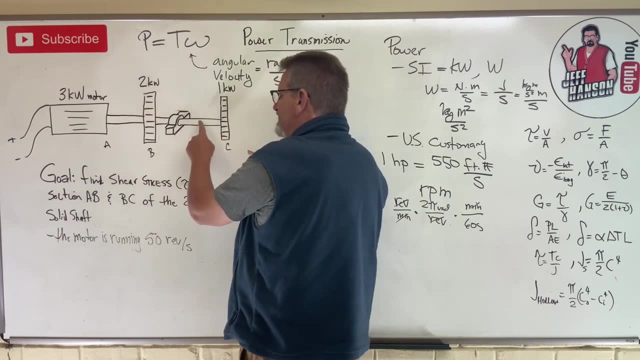 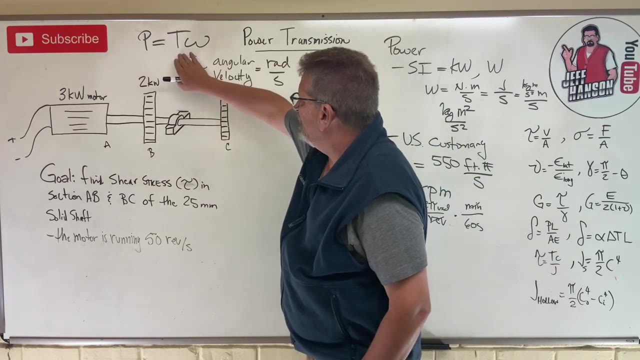 two kilowatts of power. But what's the shaft doing? Shaft AB is having to deliver power to this guy and that guy, right, But shaft BC is only delivering power to this guy over here. okay, So let's see if we can get this right. If P equals T times omega, then T must equal. 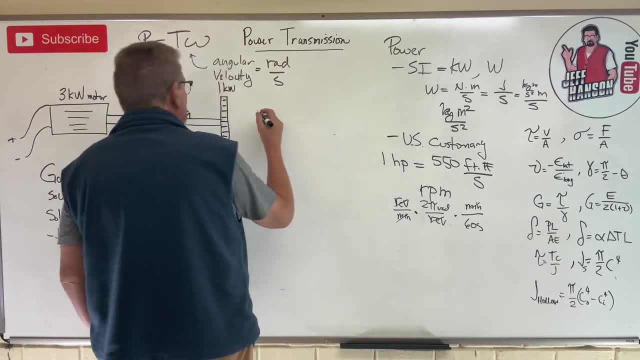 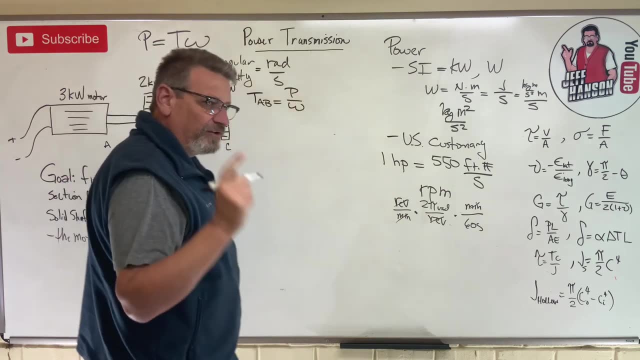 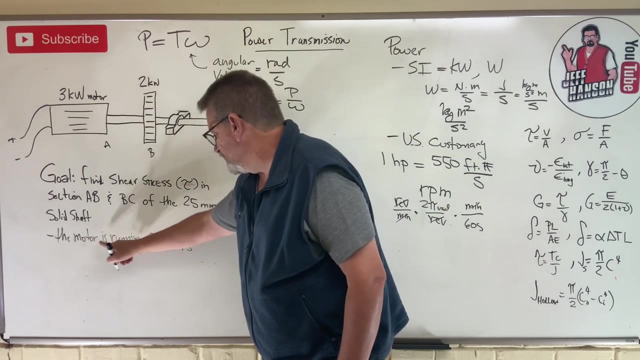 P divided by omega, Right, So T AB must be P divided by omega. Now, what is omega Radians per second is what I need, right, I need that. But what does it tell me? The motor is running 50 revs per second. 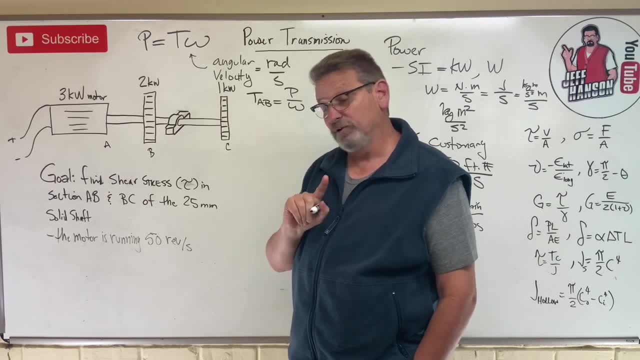 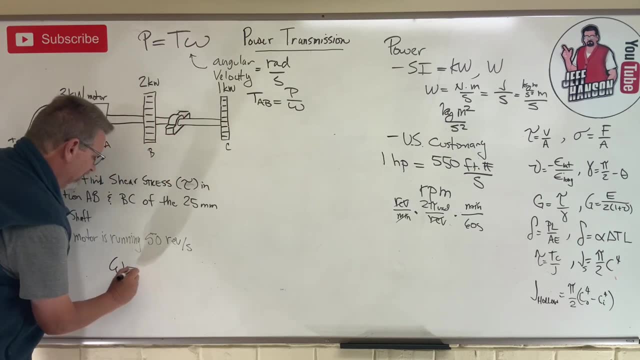 That's close to radians per second. At least it's not revolutions per minute. We've got to convert that, don't we? Okay, so omega is equal to 50 revs per second, but I'm going to get rid of revolutions. 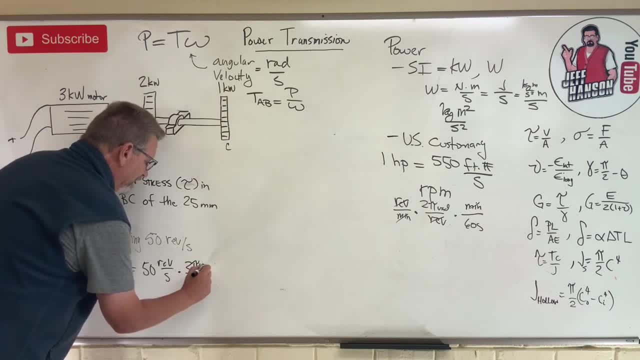 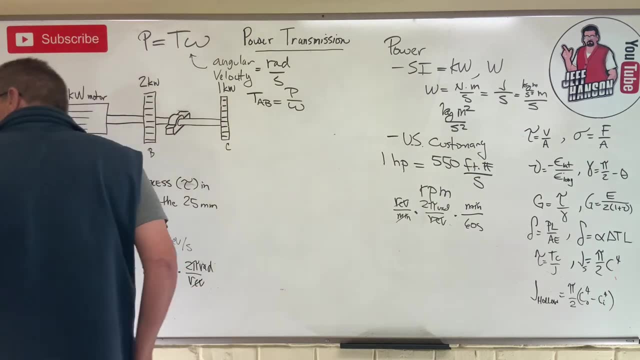 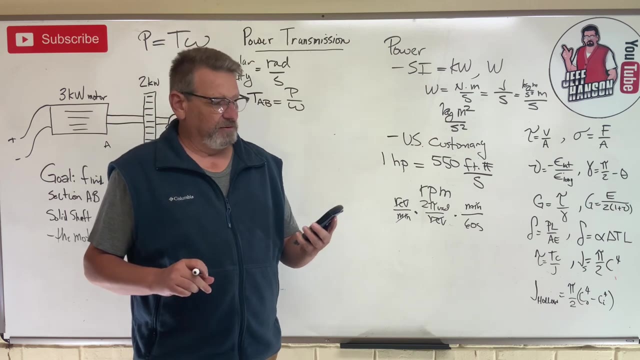 right Divided by 2 pi radians and my revolutions cancel out. That's going to leave me with radians per second. Where's my calculator? I saw one of your comments and the comment said: hey, every time, Hanson, we'll make a drinking game. Every time, Hanson. 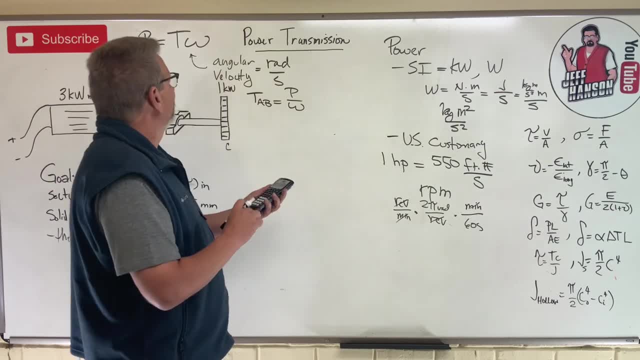 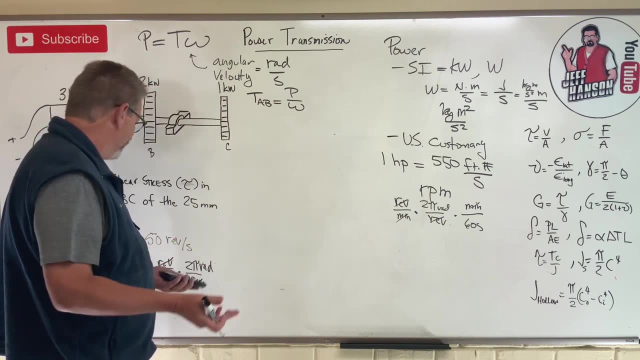 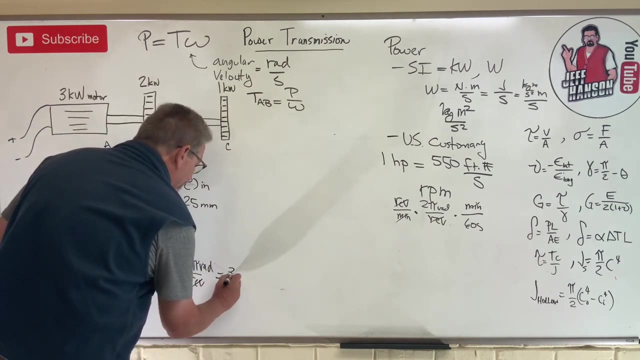 loses his calculator. you got to take a drink. Yeah, calculator. Okay, here we go. What do we got? 50 times 2.. Oh, that's why did I need my calculator for that? 50 times 2 is 100, times pi is 1. 314 radians per second. Okay, 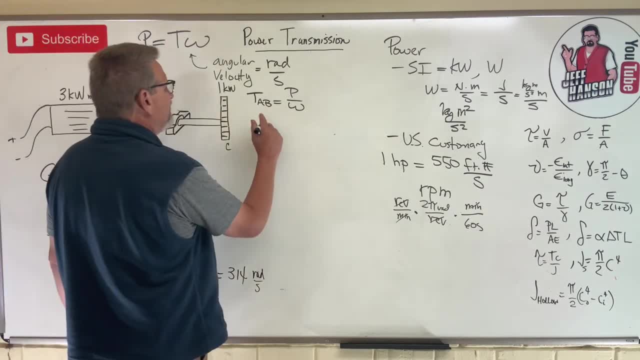 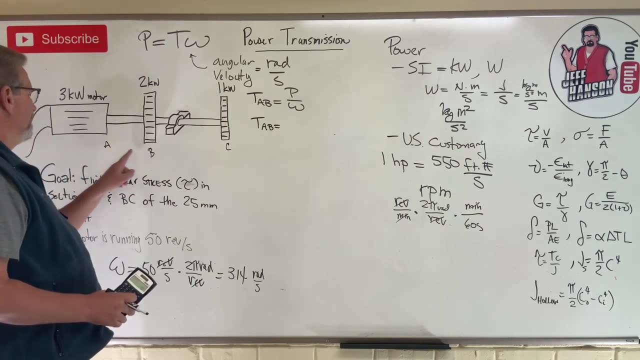 I didn't need the calculator for that, but I'm going to need it here in a minute. Okay, so T, AB. okay, the torque in section is the power in section a, B, which is what? three kilowatts, but can we just put. 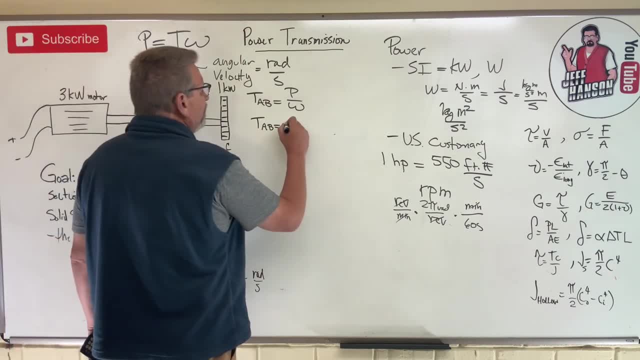 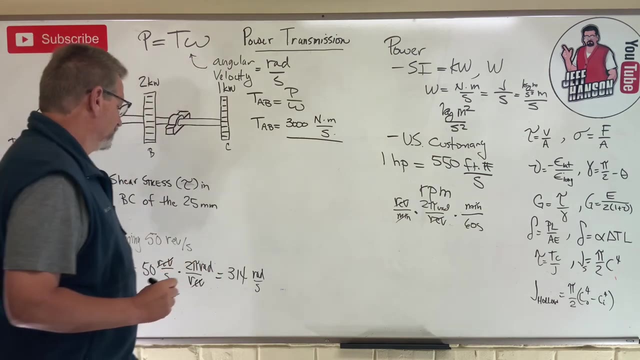 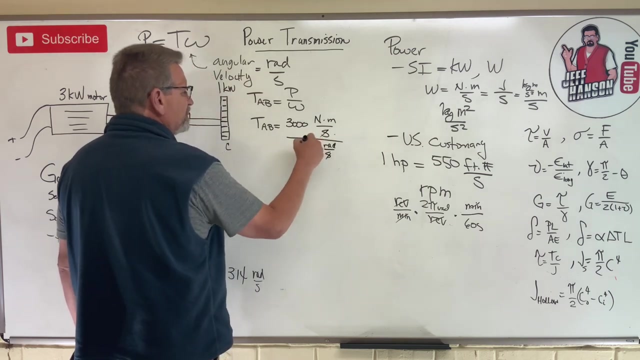 it in watts, right? so let's talk about 3,000 watts, which is what a Newton meter per second, right divided by Omega, which is 314 radians per second. so guess what the seconds are gonna cancel out? the radian is kind of a unitless thing there. 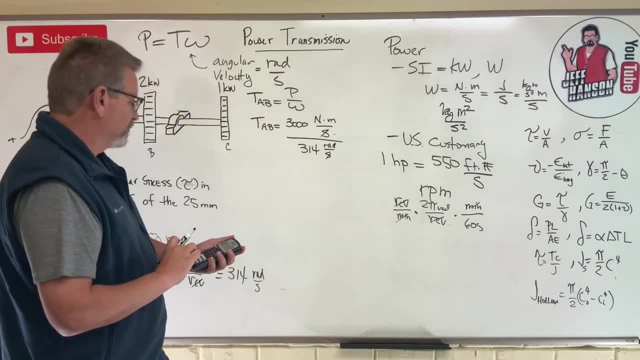 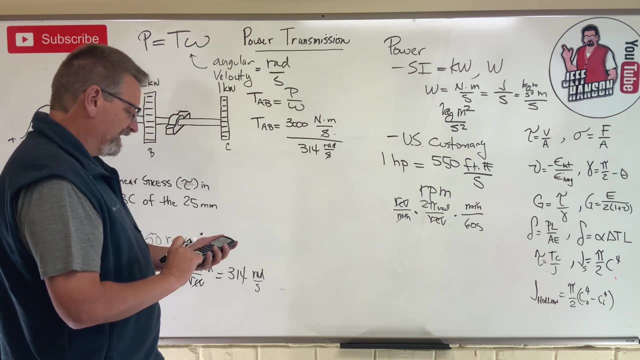 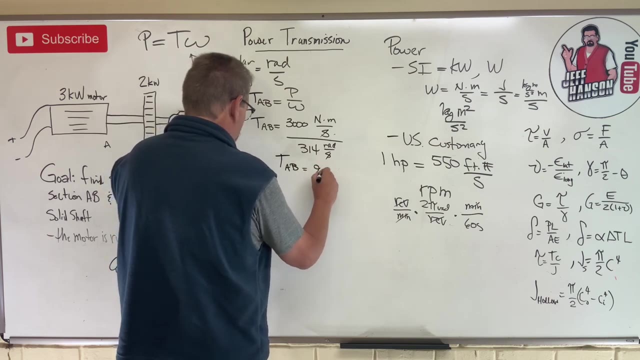 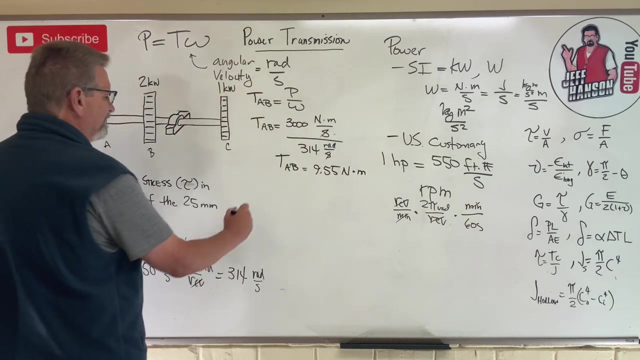 and it's gonna leave me with torque in Newton meters, which that's good stuff, right. so clear: three thousand divided by 314 equals T AB. the total of the power in section a is 314 watts, and we'll talk about that in a bit. torque in shaft ab is equal to 9.55 newton meters. okay, okay. now how about t b c? 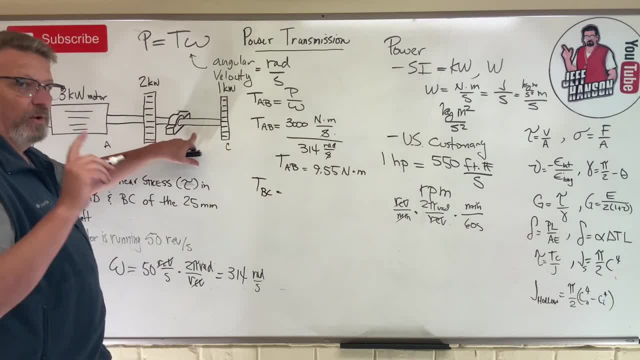 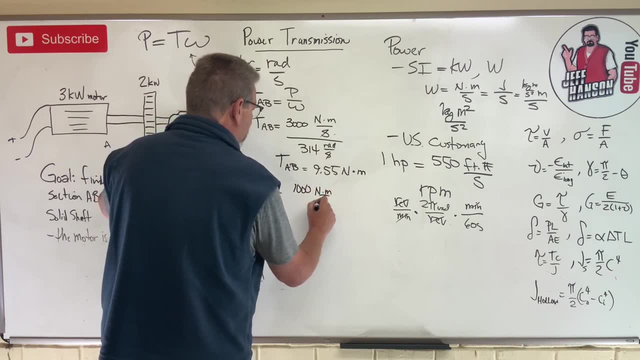 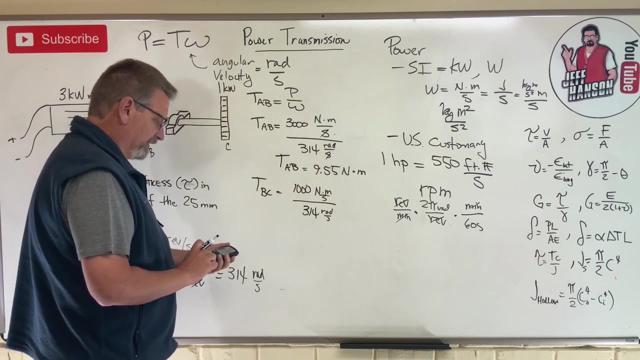 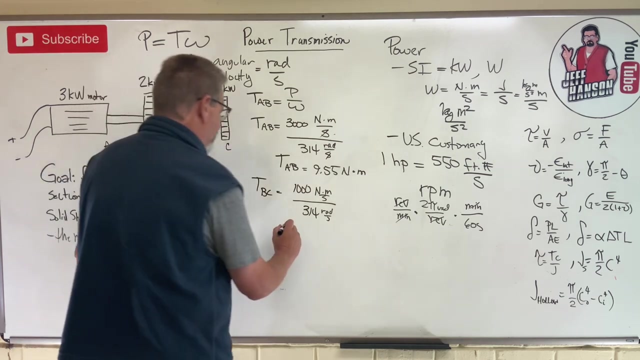 okay, what is the power over here? well, it's only one kilowatt, which is going to be one thousand uh newton meters per second, divided by the same angular velocity, right, 314 radians per second. so one, oh clear 1000 divided by 314, 3.18. okay, so t b c equals 3.18. 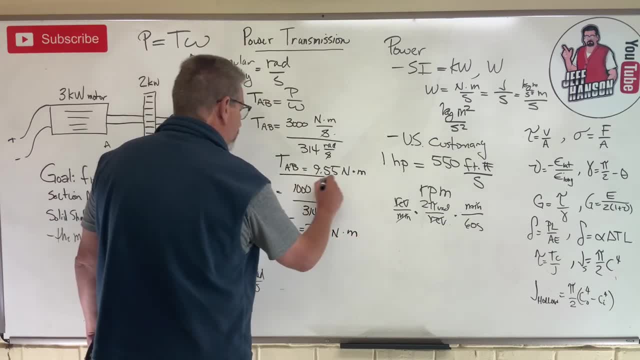 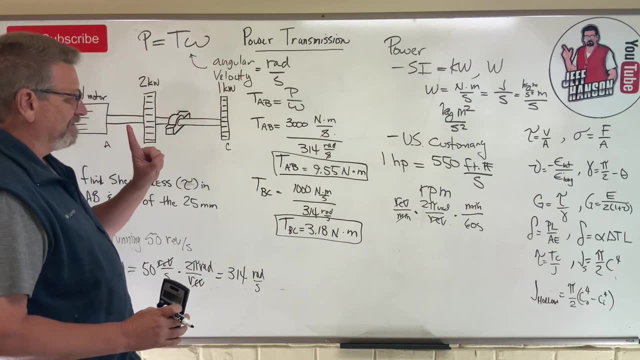 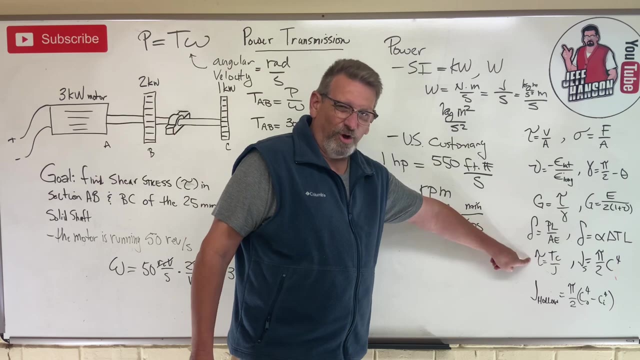 newton meters. okay, so there's the torque in both sections of the shaft. now we're not there yet, right, because we're still headed towards this. we're trying to find shear stress in each section of the shaft. but i think we're almost there, aren't we? okay? um, can we off to the side? can we go ahead and 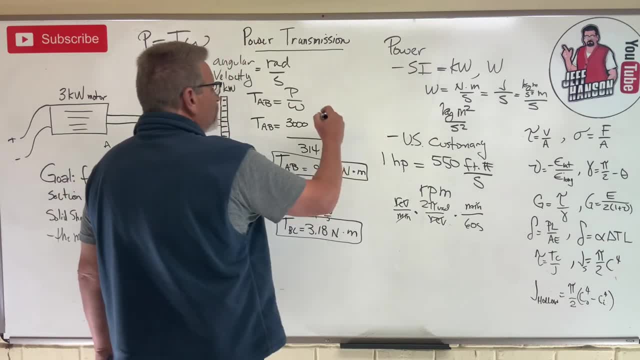 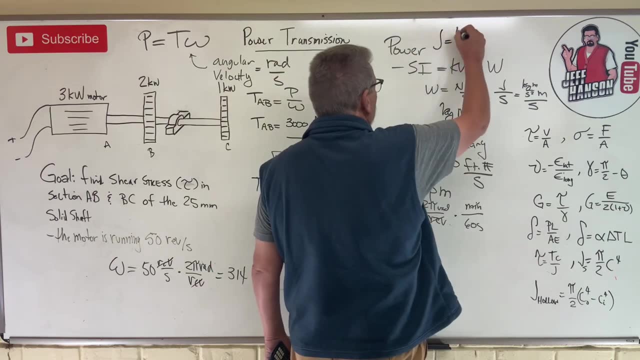 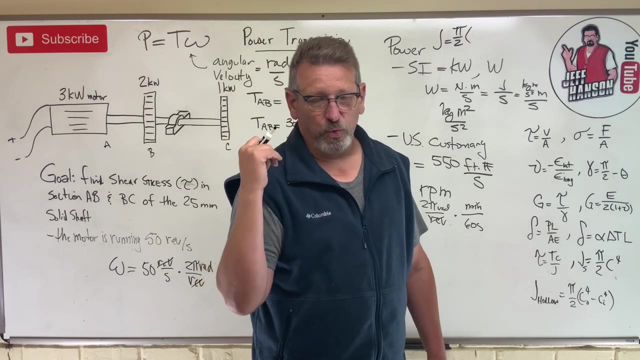 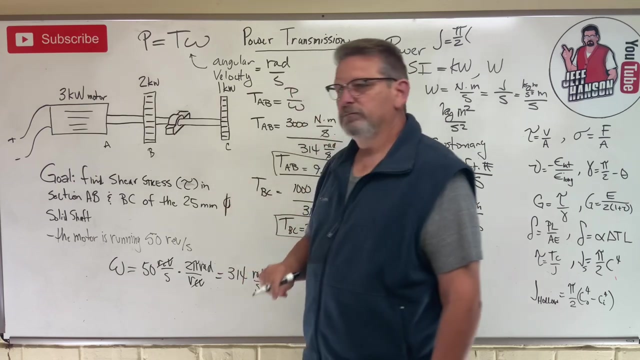 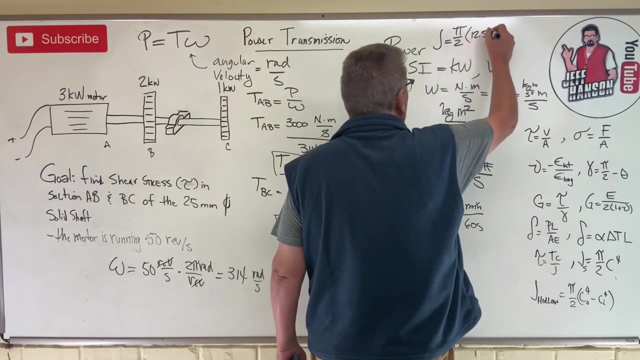 calculate j. does that be okay, if we do that. so what is that? let's see, j is equal to what here? it is right here: pi over two times c to the fourth. and what is c for a 25 millimeter diameter shaft? okay, c is 12.5. it's the radius. okay, so 12.5 to the fourth. okay, all right, let me see if i can do this. 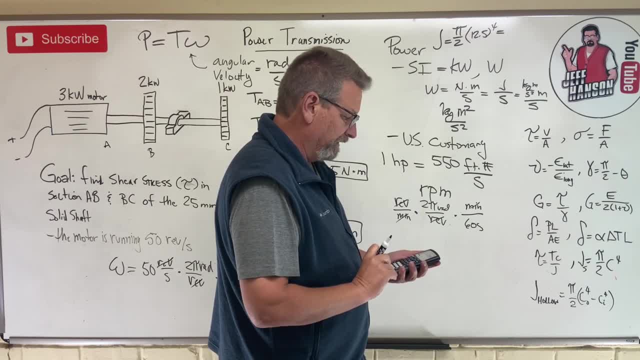 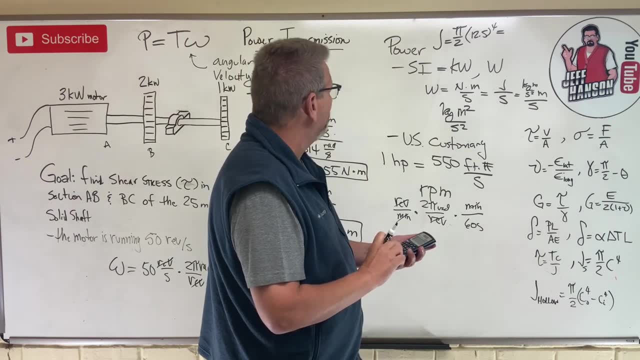 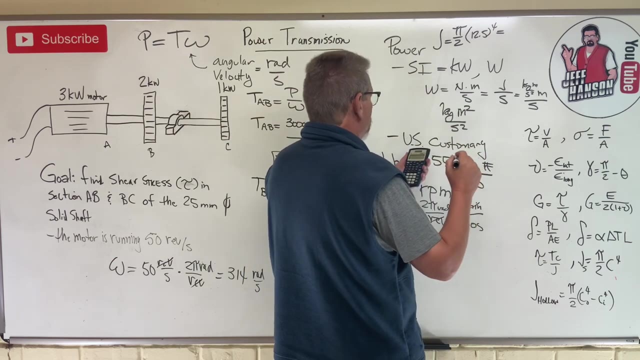 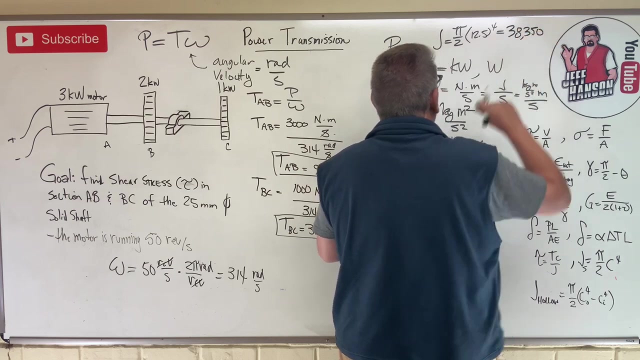 okay, so 12.5 to the fourth power is a big number, and then times pi and then divided by two is 38, 349.. let's call it 38, 350.. okay, and what's the units on that? on j, because what did i do? i took millimeters and i raised it to. 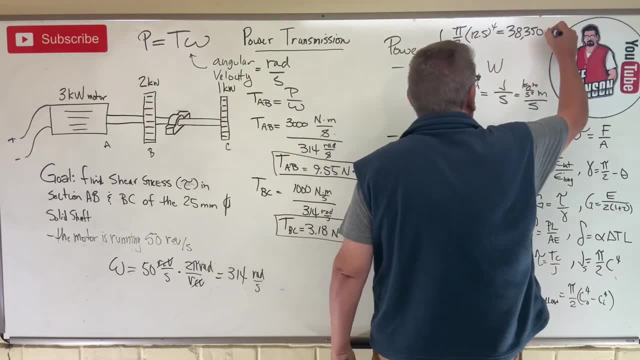 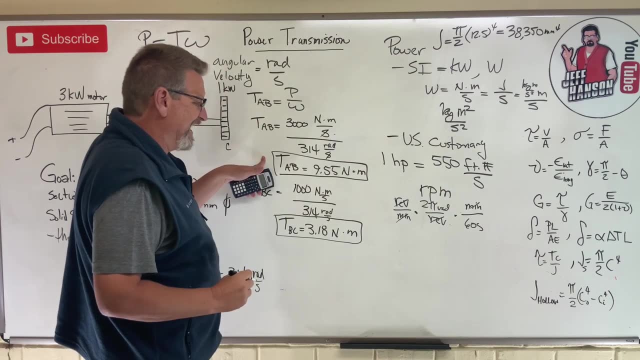 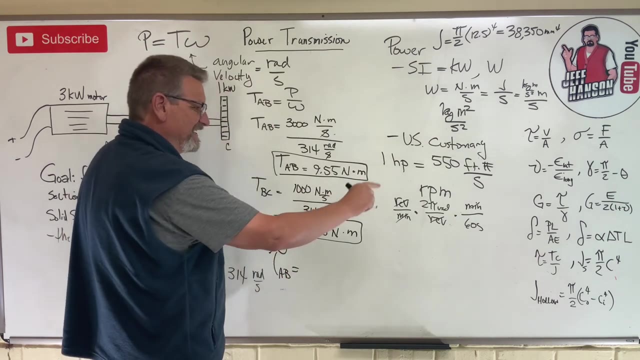 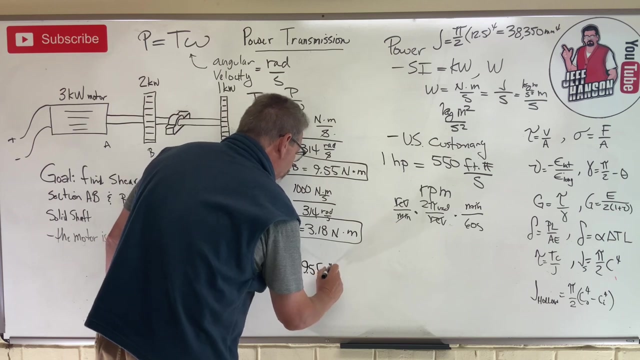 the fourth power. so that's millimeters to the fourth, okay, mm to the fourth, okay. so here we go. let's start with this guy. let's find a b first. so here we go. tau, a b is equal to t c over j t, right there: 9.55 newton meters. now, everything i have is in millimeters. i think we ought to get rid. 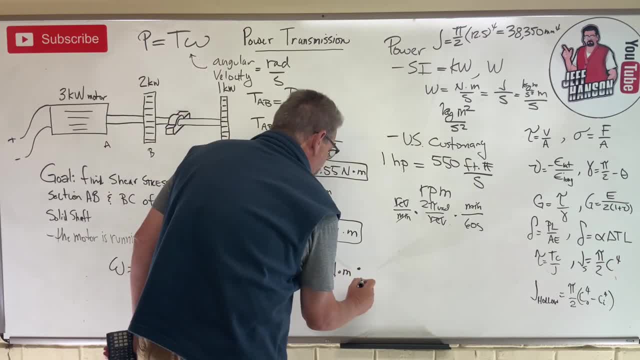 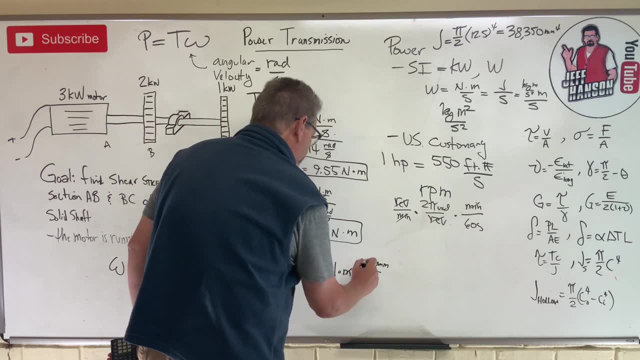 of that, meters right there. so let's go ahead and just do this. let's do: that's a meter on the top, so let's put a meter on the bottom and that's 1000 mm. okay, get him out of there and then times c right t. 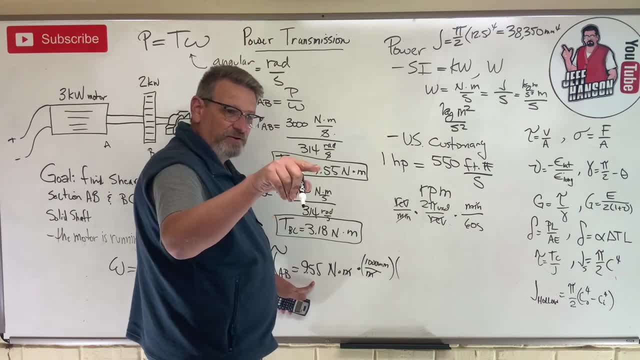 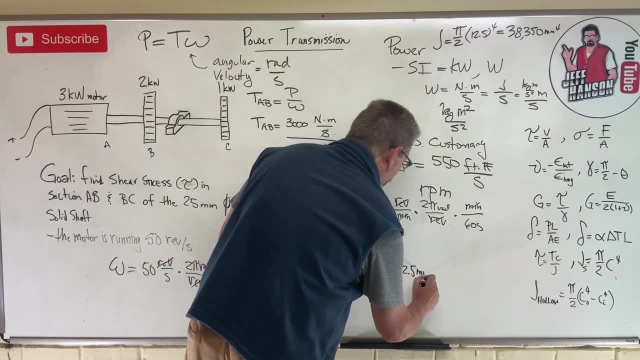 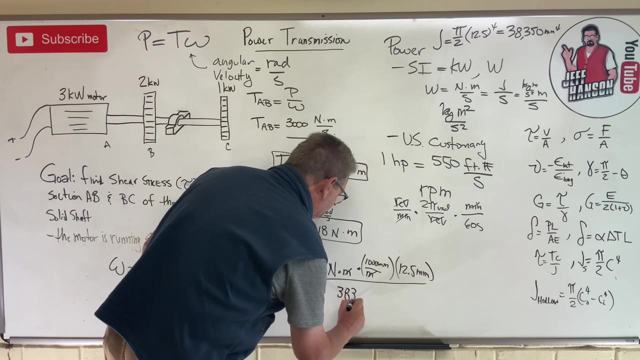 c over j. c is what? from the center of the shaft to the outside of the shaft, which is a radius which is 12.5, okay, divided by j, which we just calculated, didn't we? 38 350 millimeters to the fourth. okay, now, what do we have? we have millimeter and millimeter, that's. 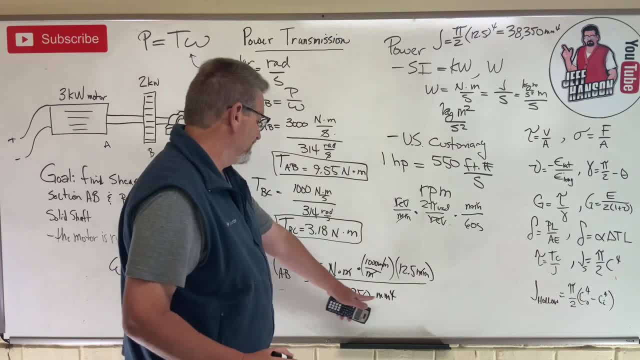 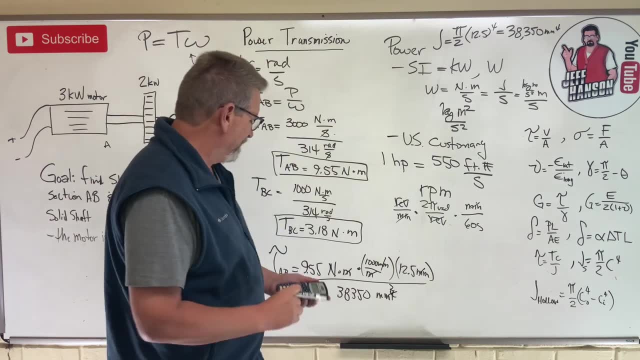 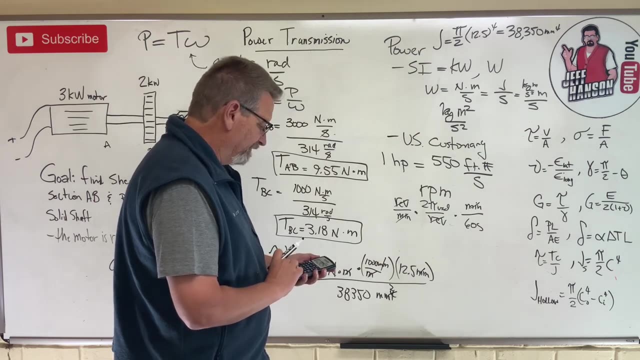 a millimeter squared, burnt, burnt. and then what is that? oh, that gets rid of two of those. so it leaves us with newtons over millimeter squared, which is what that's? a mega pascal, isn't it? so here we go: 9.55 times, 1000 times 12.5. 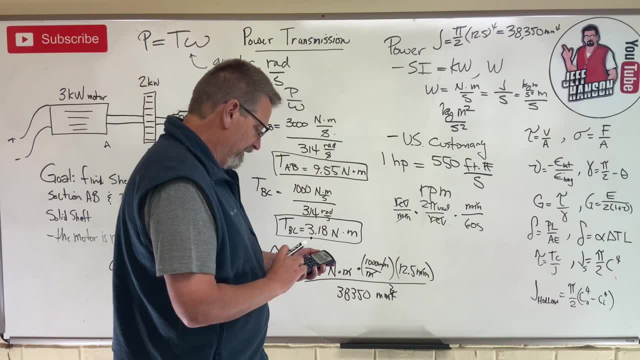 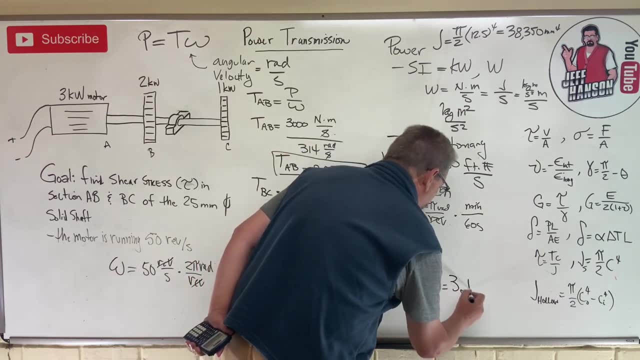 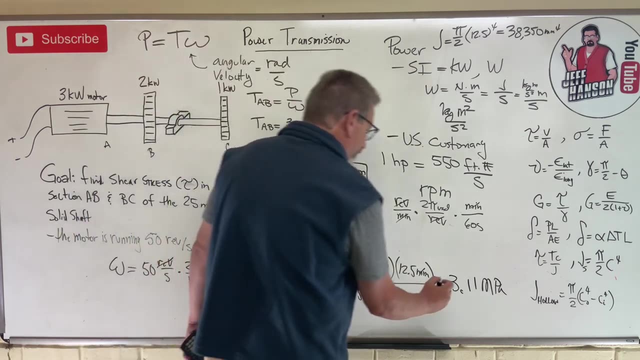 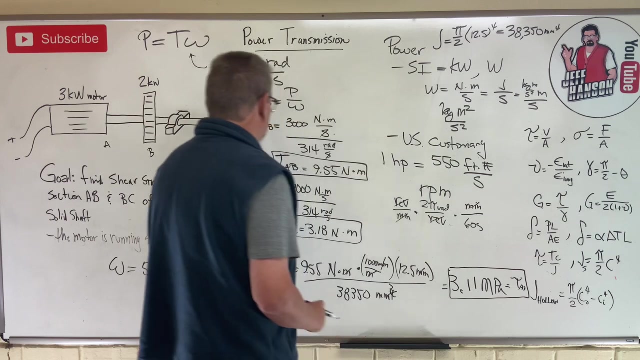 equals. divided by 38, 350 equals 3.11. how is that? 3.11 mega pascals. okay, that is the answer for tau a b equals tau a b. okay, that's one of the answers i'm looking for now what about the other one? let's make this a little a. 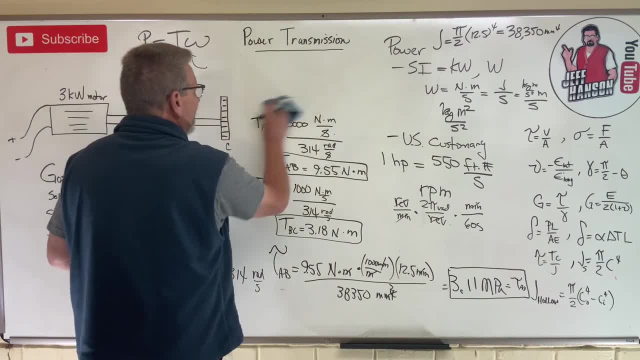 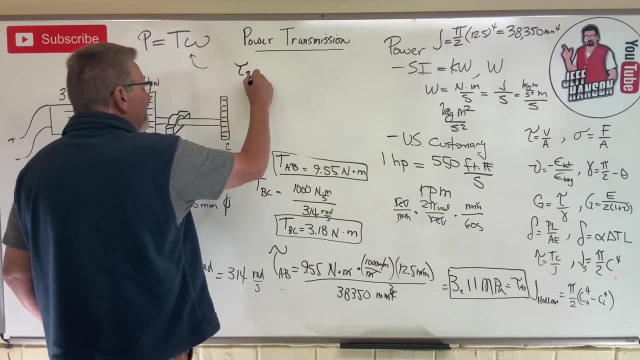 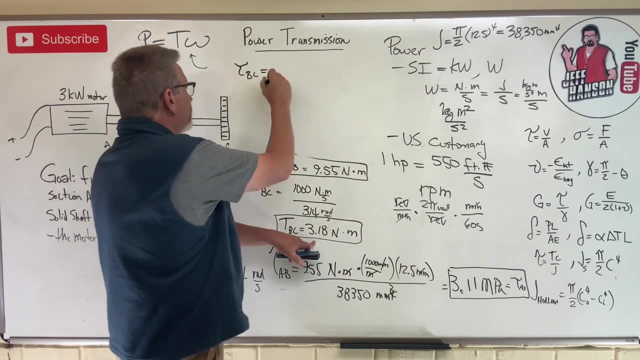 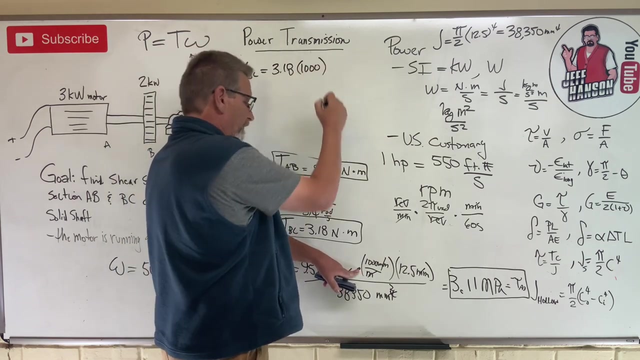 bit of room up here and see if we can get the last one. okay, tau b, c is equal to just like we did down here, right, it's equal to- there's the torque in that section- 3.18 times a thousand. i'm doing the exact same units, right, so i'm not around my units times. 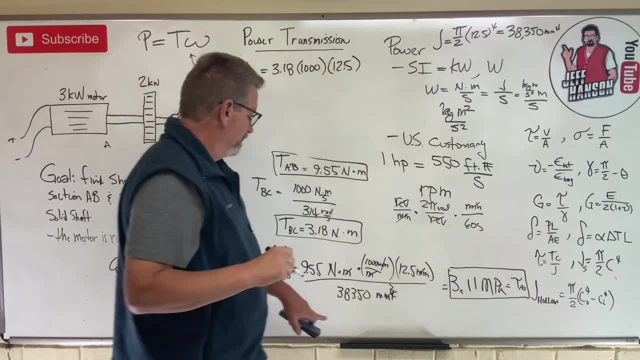 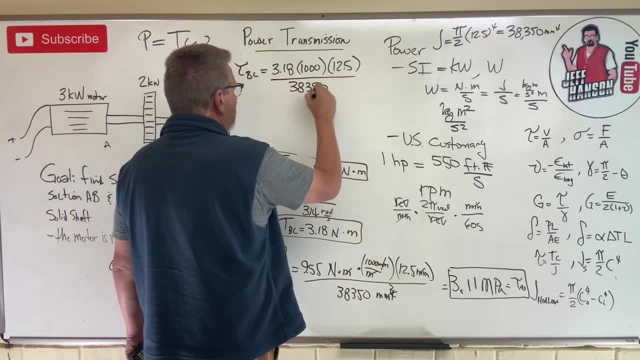 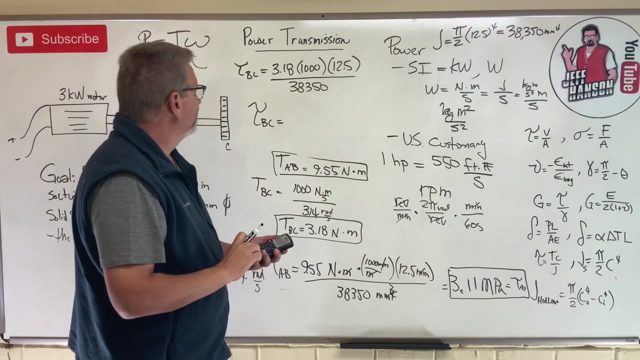 c 12.5. same diameter is j. the same j is the same. divided by 38 350, therefore, tau bc is equal to- here we go, 3.18 times 1000 times 12.5: equals divided by 38 350 equals 1.04.